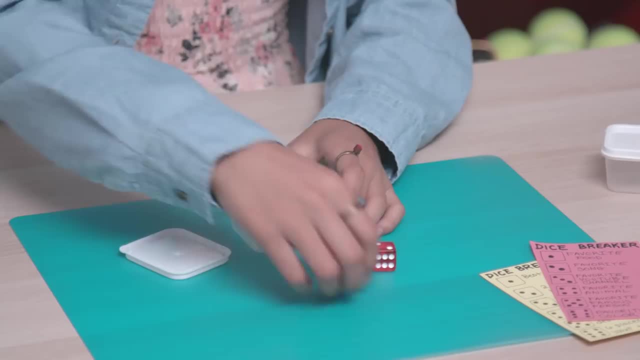 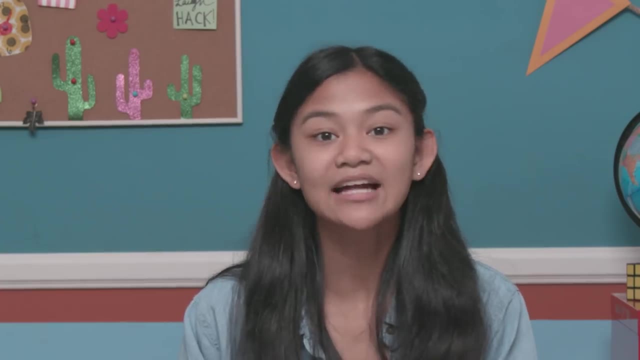 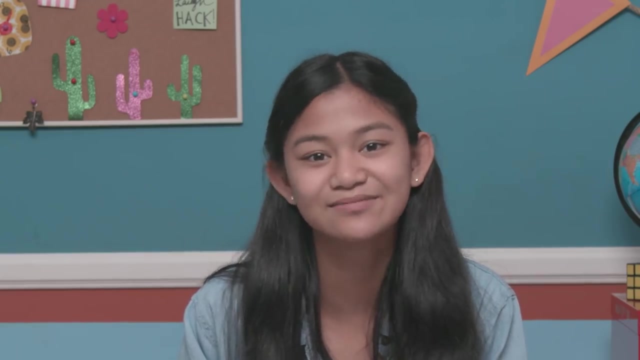 Now place one of the dice in each of the containers and put on the lid To play. hand out a box and a card to a new friend. Each of you takes a turn rolling your dice and answering the questions based on the number it lands on. 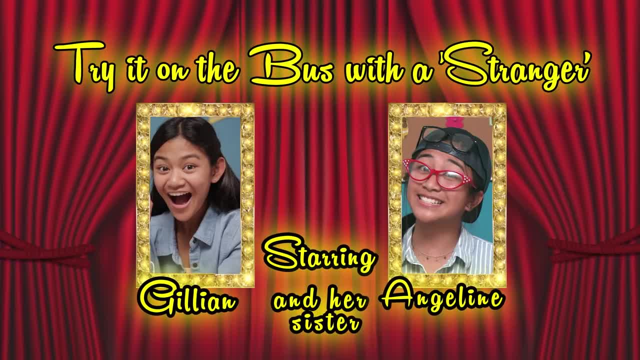 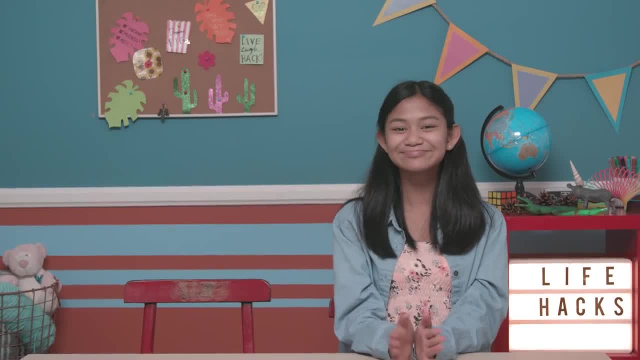 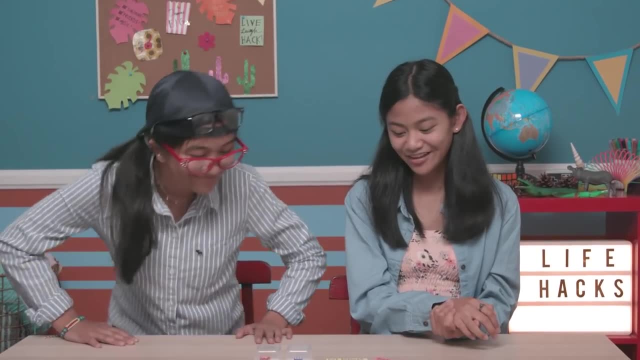 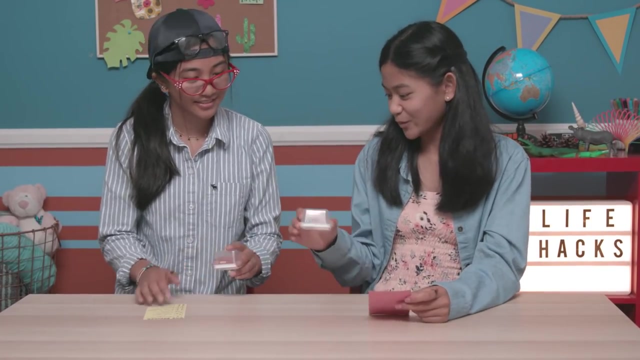 Here I am riding the bus all alone. Is this seat taken? No current, stranger future friend, Have a seat. Want to play a game? Sure, Take a card and take a dice. So roll the dice first. 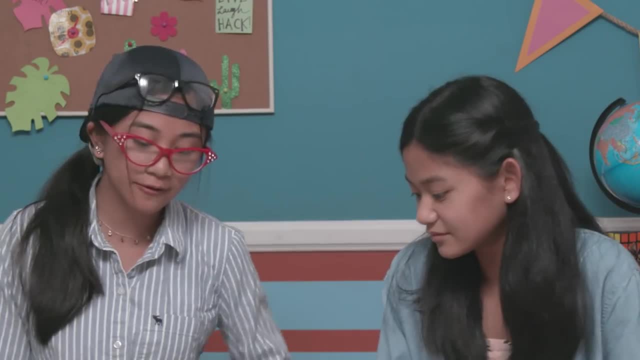 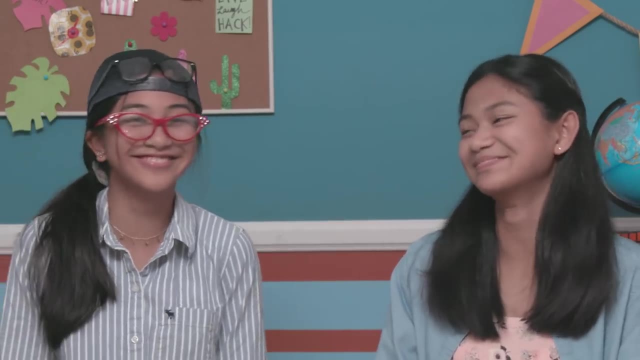 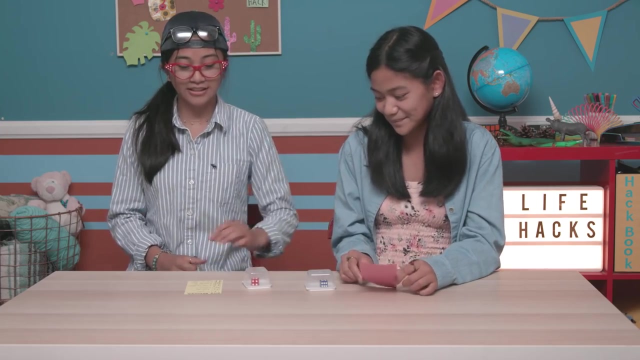 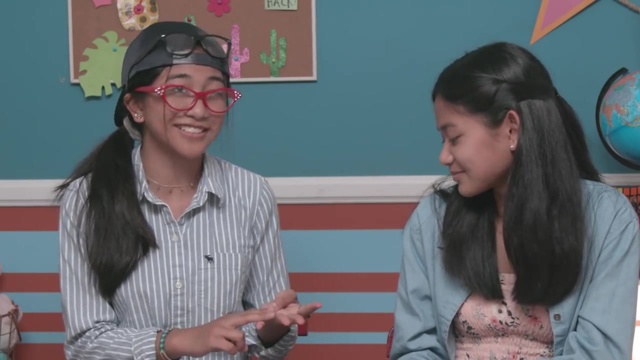 What did you get? Two of your favorite hobbies: Singing and drawing. Favorite color: Blue. Do you want to go again? Yeah, Five, Five words that describe you: Fun, Creative, Funny, Intelligent, Nice. One Favorite food. 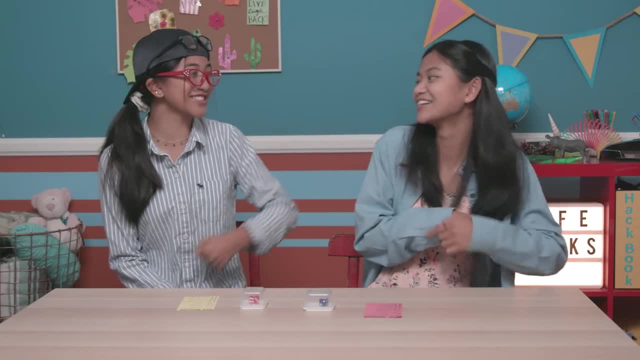 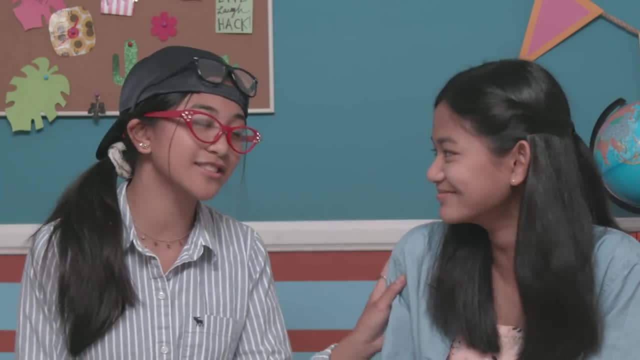 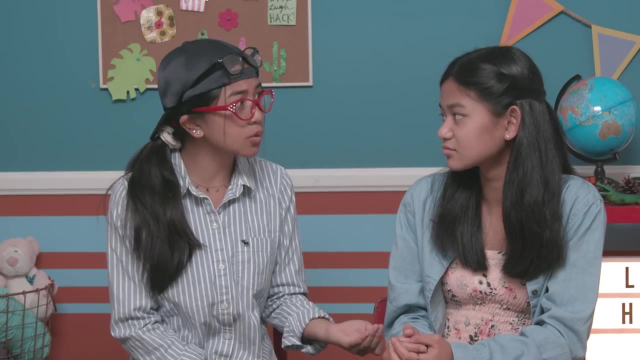 You too stranger, You too stranger. Now that we're new friends, I feel like I can confess to you I get really stressed riding the bus. I keep worrying: are we going to get to school on time? What's for lunch today? 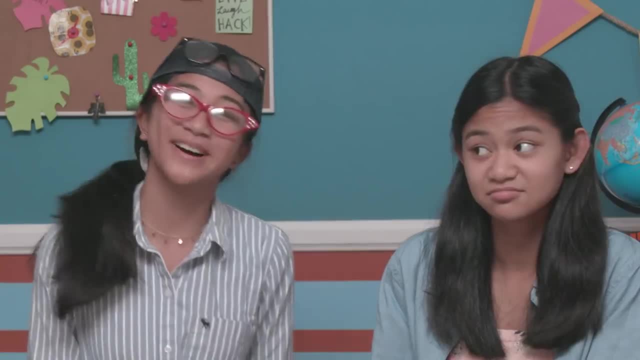 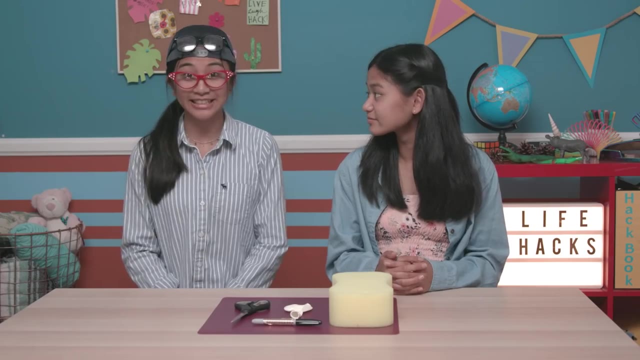 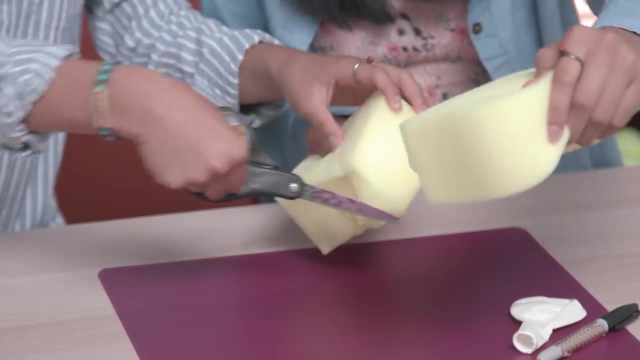 Did I forget a history course again? But thanks to this hack, I can turn bus time to zen time with a super squishy. For this you'll need a big sponge, a white balloon, a black marker and scissors. Take the scissors and cut the sponge into the shape of a circle. 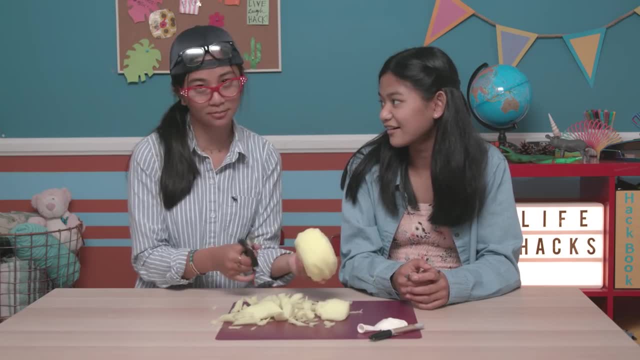 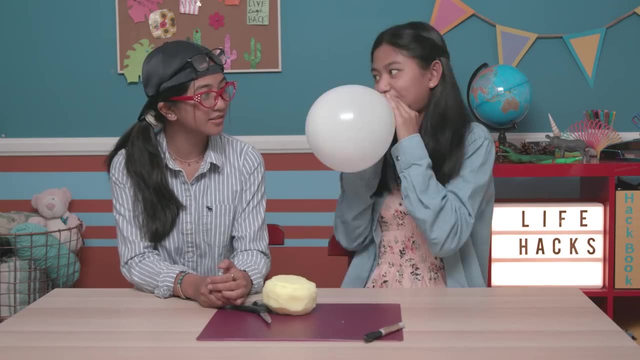 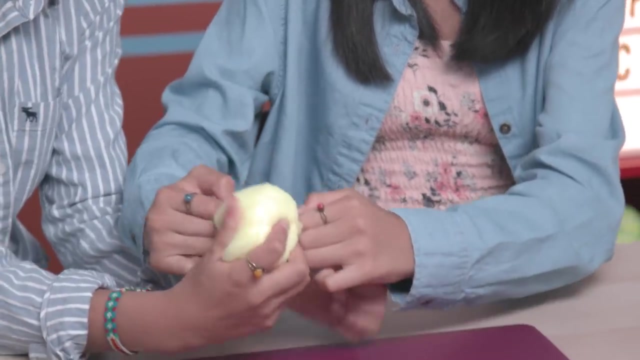 It kind of looks like a burger. Great, now I'm hungry. Now blow up a balloon as big as you can and let the air out. Now cut off the mouth of the balloon and stretch the whole thing over the sponge. Tuck the end of the balloon in like this: 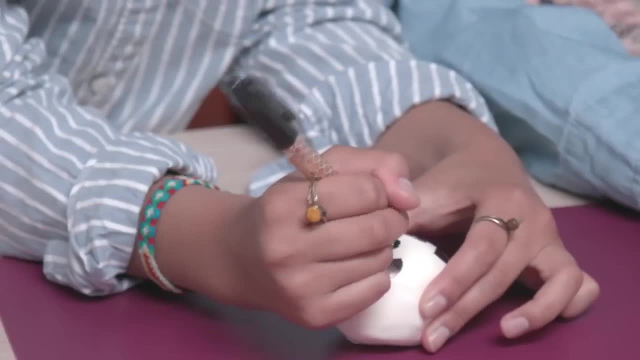 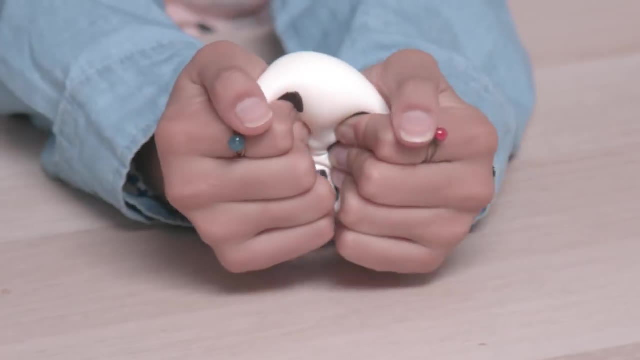 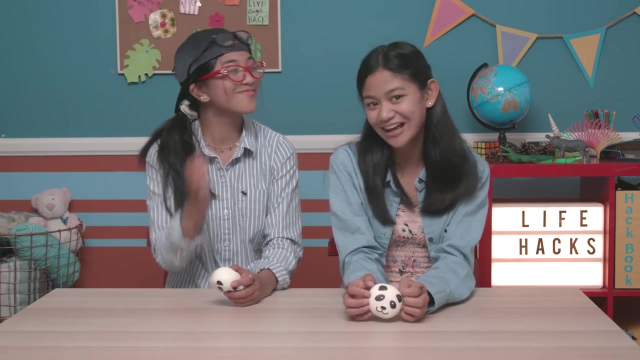 Don't seal it because it still needs to let air in and out. Draw on a face. It's time to squish away, Squeeze in, chill out. Great hack, new friend I never met before today. And finally this last hack can make the bus ride fly by. 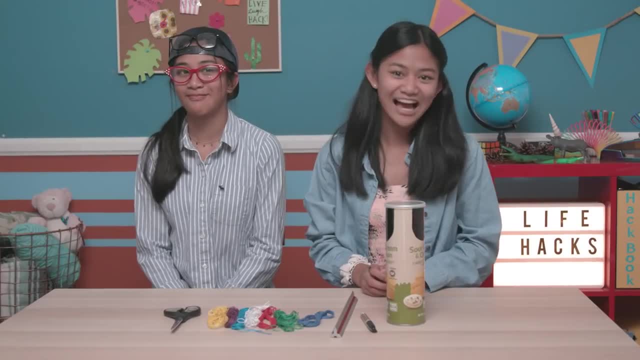 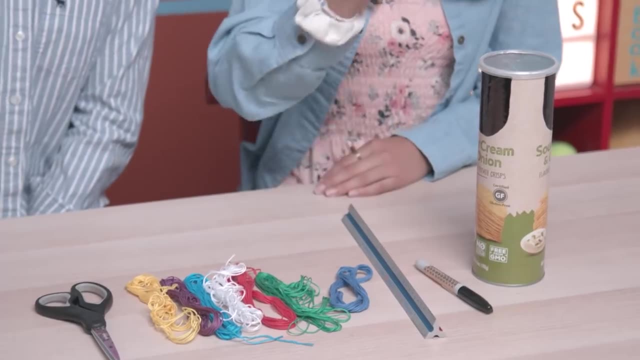 My friendship bracelet to go, My friendship bracelet to go, My friendship bracelet to go. For this hack you'll need scissors, seven different colors of embroidery, floss, a ruler, a permanent marker and a potato chip. can Draw four lines on the lid using your ruler, like you're cutting up a pie. 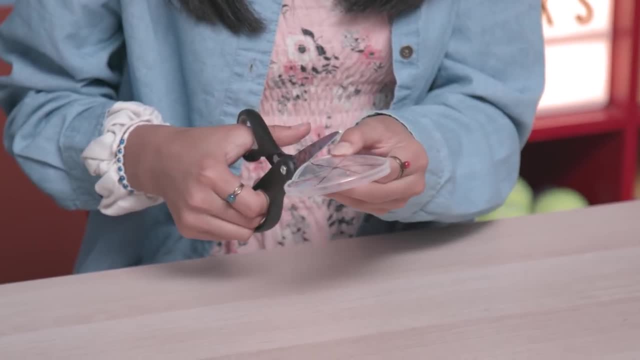 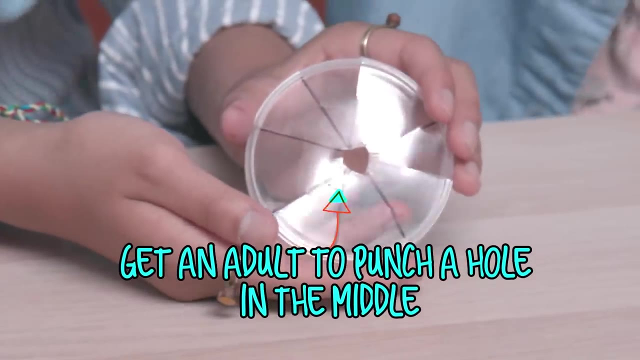 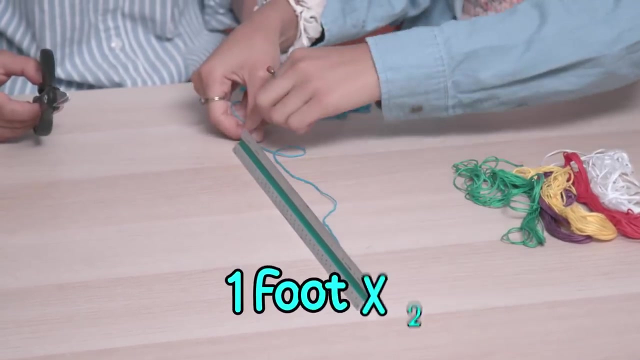 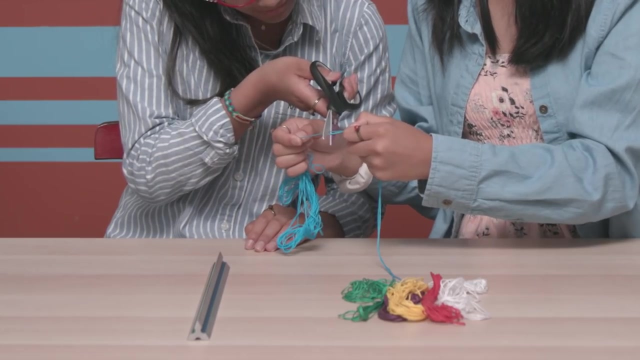 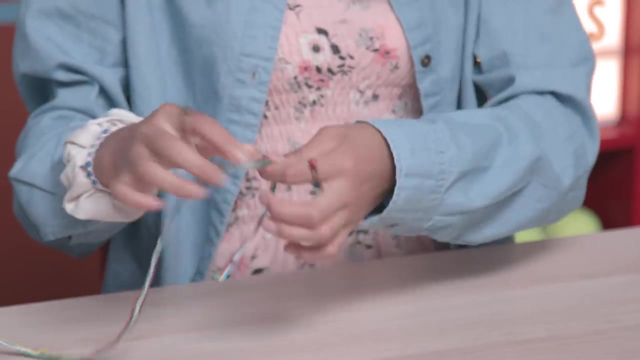 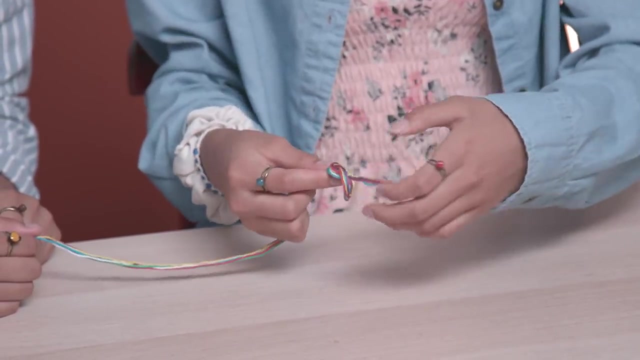 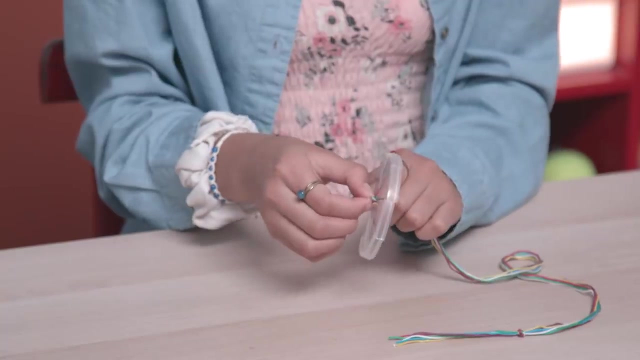 Cut a half inch up each line. Cut a two foot piece of each color of thread. Tie a knot on one end of your strings. Leave about three inches of a tail restoring. Put the ends of the string through the hole in the lid. 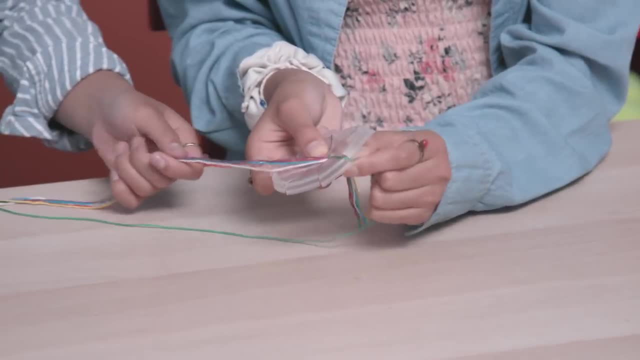 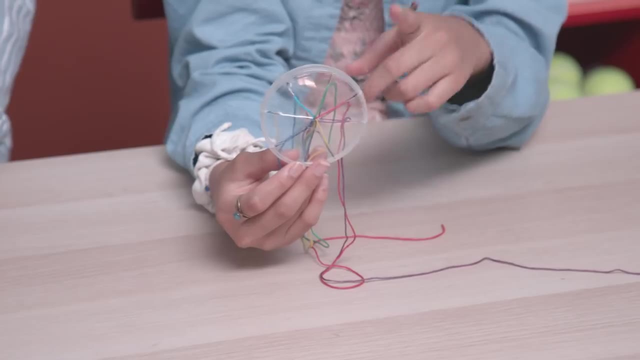 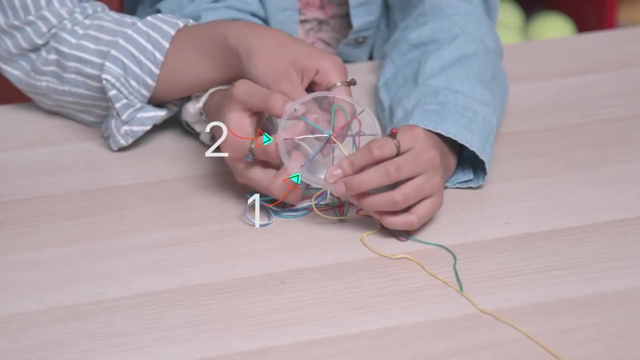 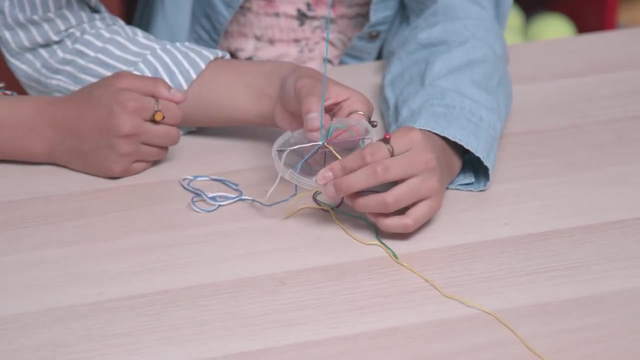 Now put one string in each slot. You have seven strings and eight slots, so one slot should be empty. Turn the empty slot to the bottom and count three threads clockwise. See three threads clockwise. Pull this thread across and into the empty slot. 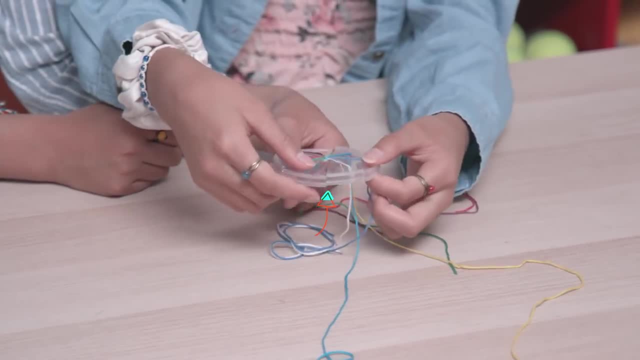 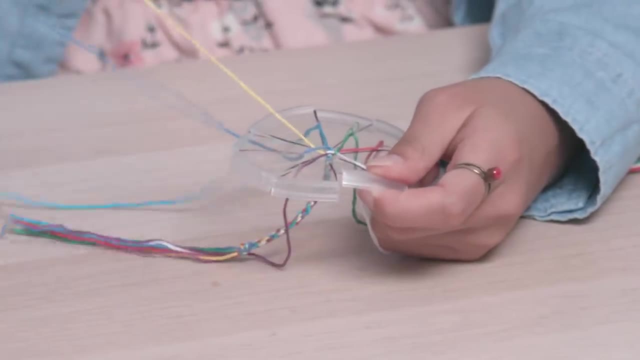 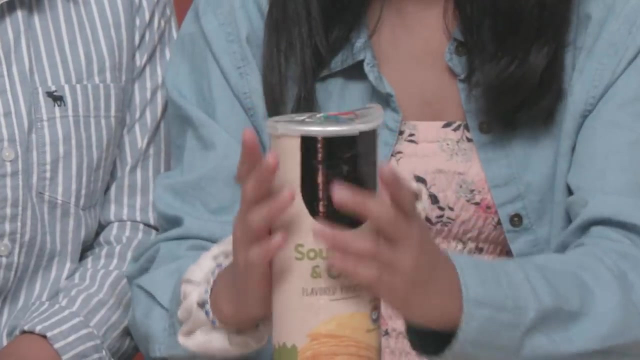 Turn the empty slot to the bottom again and repeat over and over As you go. gently pull the bracelet through the hole, Keep going And you can always replace the lid on the can when you get to school and keep working once you're back on the bus. 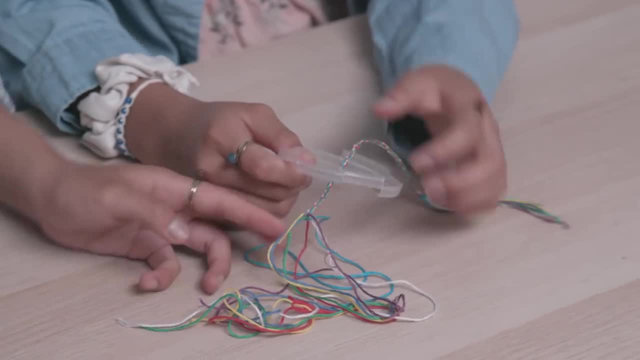 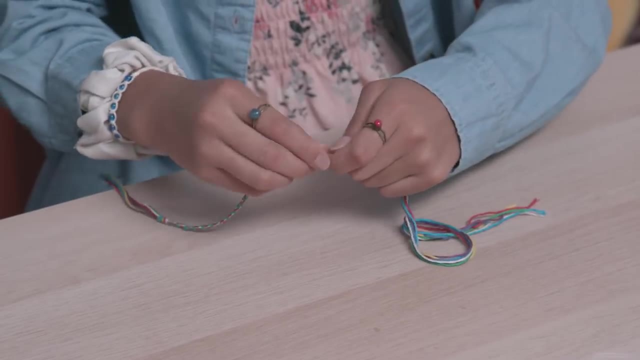 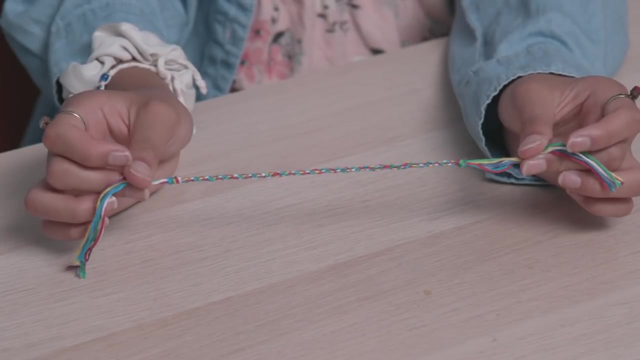 Once the bracelet is long enough for your wrist, like it is for mine, remove the threads from the slots and pull the ends through the hole. Tie another knot at the end and leave yourself a three inch tail. That looks great, Can I have it?